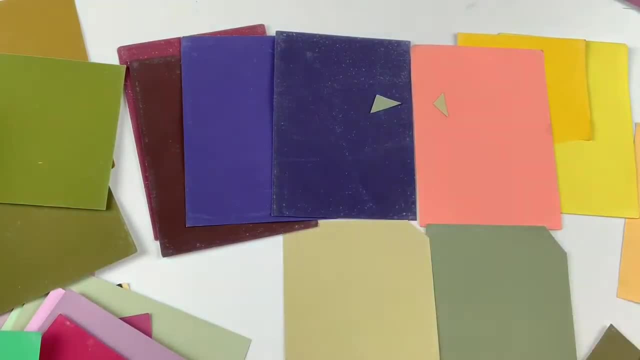 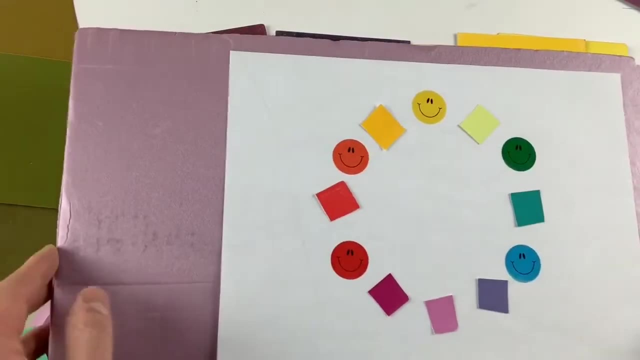 color you need to consider. There's hue, there's value and there's intensity. Okay, So hue is the name of the color. The first thing we're going to talk about is this amazing color wheel I quickly made because I don't. I have limited resources at the moment and I had to put something together. 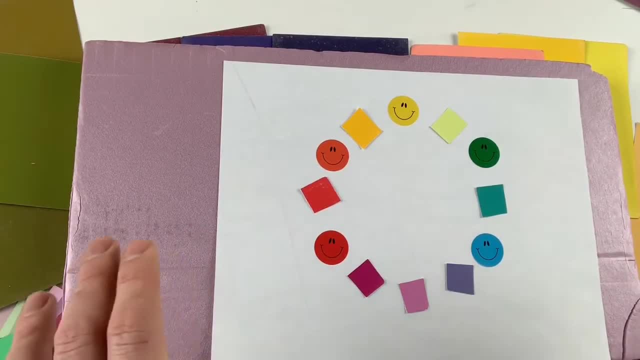 so I can explain a few things. The name of the color is related to hue. Hue is the name of the color And when we talk about that, it's a 12 hue color wheel. In terms of colors like Midnight Blue or Crimson, Tide Red or colors like that, they do not exist in a color wheel. That's not the language. 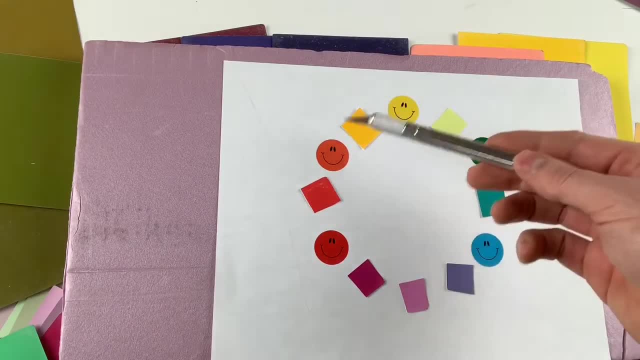 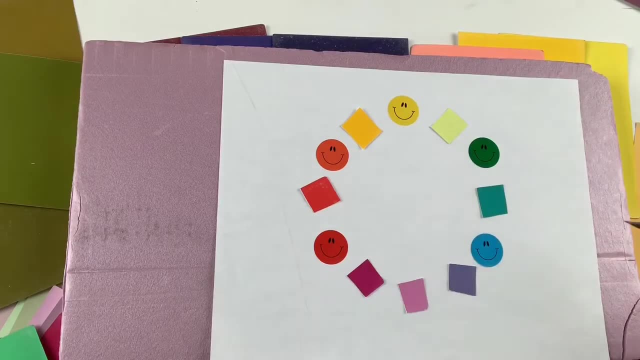 that we're going to use, The language that we're going to use, is yellow, yellow-orange, orange, red-orange, red, red-violet, violet, blue-violet, blue, blue-green, green and yellow-green. That's. 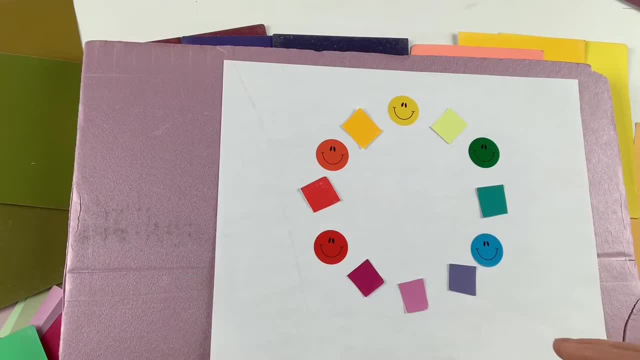 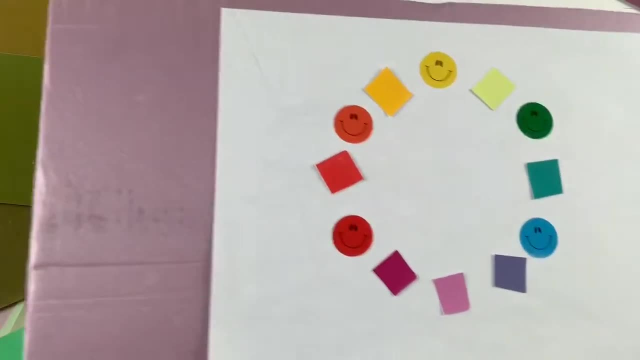 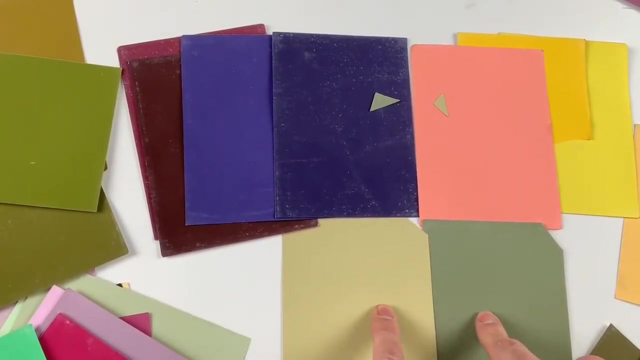 it Twelve hues and everything related to color. That is reference to this color wheel when we're talking about hue. All right, So the first thing we want to distinguish is what's the difference between these two? And the first clear difference is hue: This is green compared to this and this is yellow compared to this. Now, if I put this, 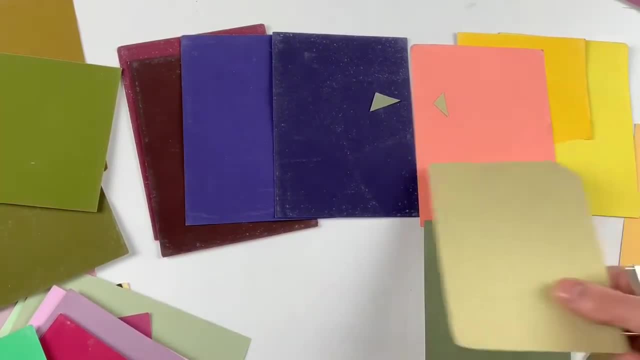 next to something else, like I put next to this yellow or this orange, it appears more green. but I'm only comparing these two colors, That's it. Another clear contrast between these two is value, So that's the second characteristic of color we're going to talk about. This is clearly darker than that, So if you took a 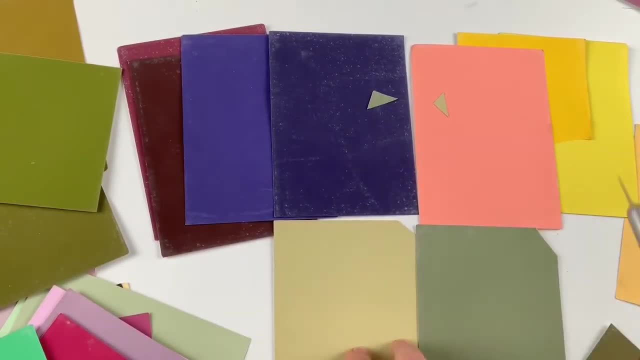 black and white photograph of these two. this is darker, this is lighter. Don't worry about we're isolating the value, We're not thinking about hue at the moment, only dark and lightness. The third characteristic of color is intensity And in this case, 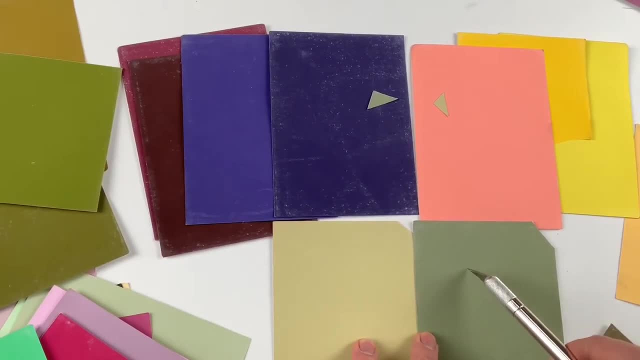 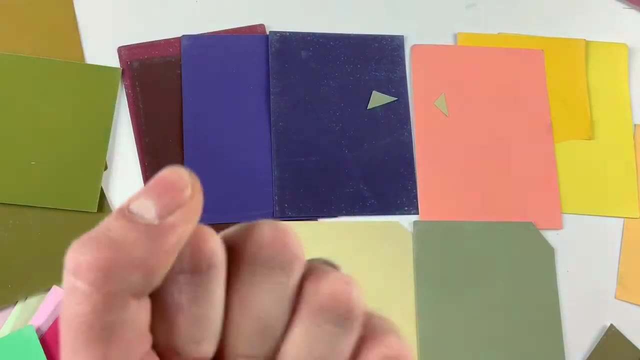 if we go to a picture of an image like this, where you look at a screen and see the slide, I would say that how I'm looking at it is well, not in this case, In all cases, when I'm referring to intensity. 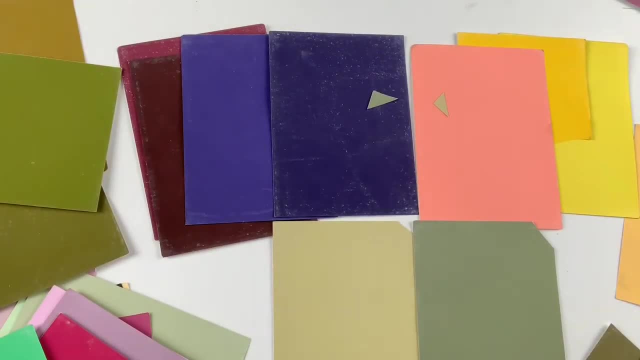 is something that is super intense compared to something that has no chroma whatsoever, in terms that it's pure gray, And think of a scale between those two. So if I were to have a very intense color, like to say this green, and then I slowly transitioned it into a pure gray, This will probably be the color I would want, okay. 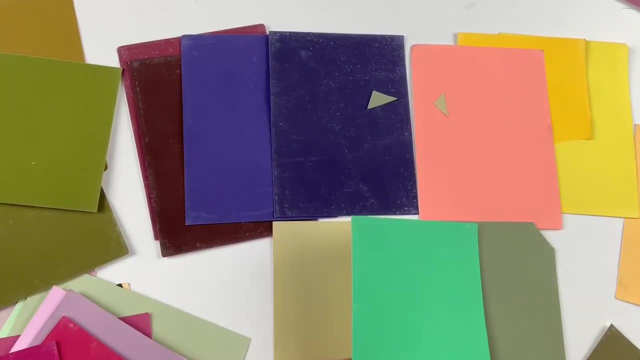 would be part of it. this would be in the middle of that transition to pure gray. so this color here- actually, I kind of have this handy dandy- this color here, this could be the the root of that color, right? so this is yellow orange and if I 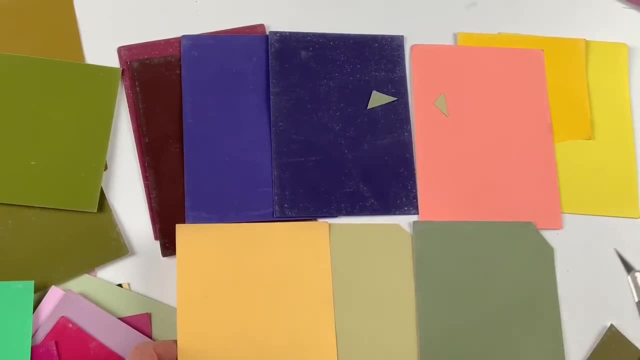 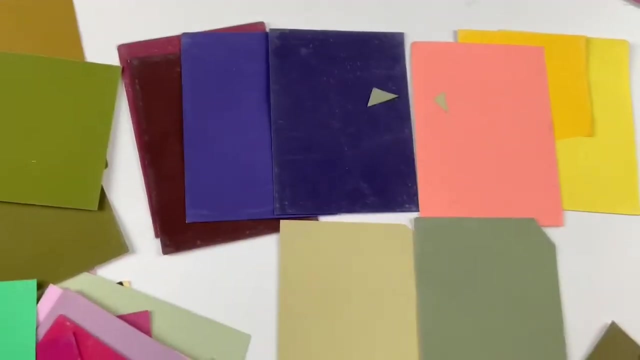 were to gray this yellow orange out, it could look like this along its way to pure gray. so, in terms of saturation levels, these are the same. if I were to, this being a number one, this being a gray being a number ten, I'd say: this is about a five. this being a number one, this gray being a number ten, I'd say: 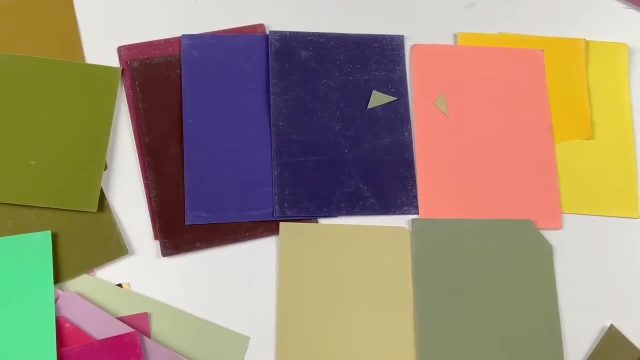 this is also a number five. it's about middle intensity level. so in this discussion, intensity is not going to be an issue. I'm not going to consider that when I'm trying to make these two colors look the same, because one is not more intense than the other. 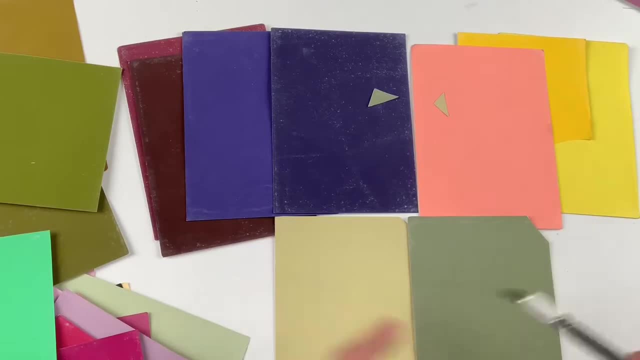 but the two things that I need to figure out is: I need to make the values look similar and I need to make the hues look similar. so the first thing, I want it, my first objective, let's talk about hues. this is yellow, this is green compared to. 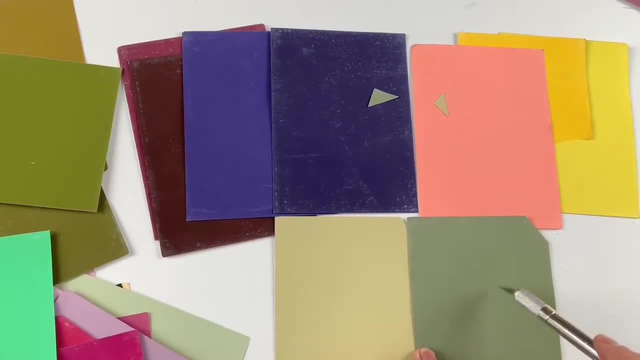 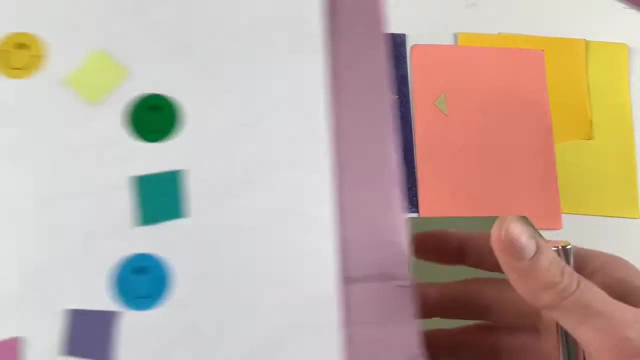 one another. I want to make this one appear green, I want to make this one appear yellow. how do I do that? I can do that just by changing the backgrounds of all the color. but in order to do that, I need to know my color wheel, and here. 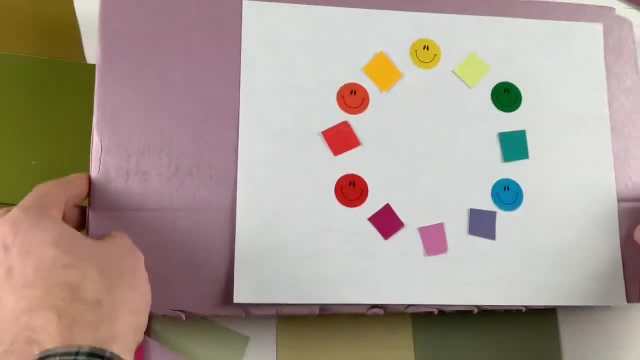 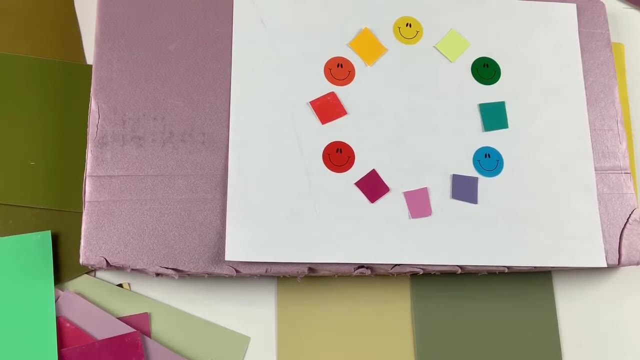 we go again with my smiley face color wheel. so if I'm trying to make a green, I'm going to move this up a little bit. this color up here, green, my objective is green, so then I go to green. I'm trying to make this look green, so I 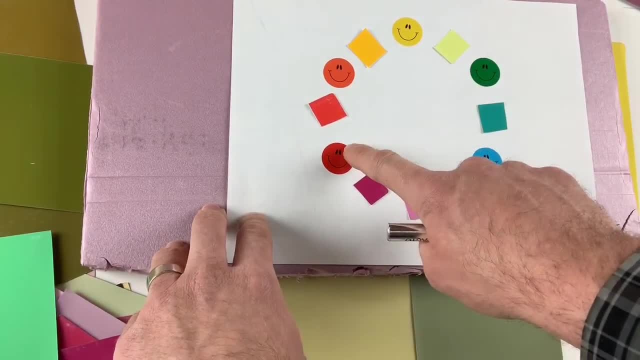 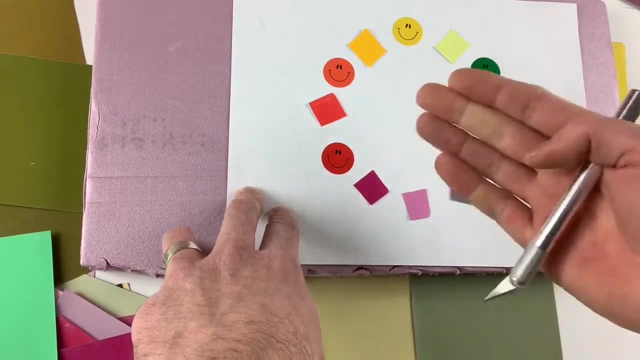 go to green, but in order to do that, I need to do the opposite of that. so then I go to the opposite side of green, which is red. now I know that red is going to work or get me in the right general direction. I'm not sure if it's gonna be. 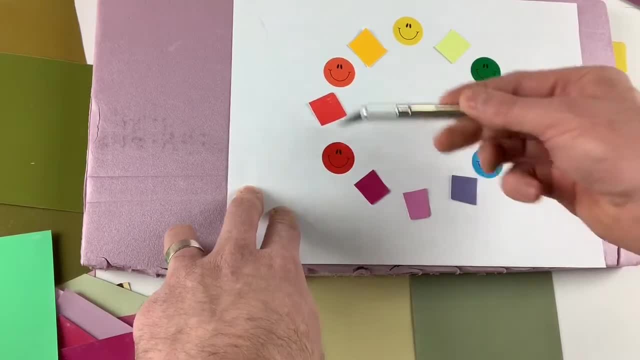 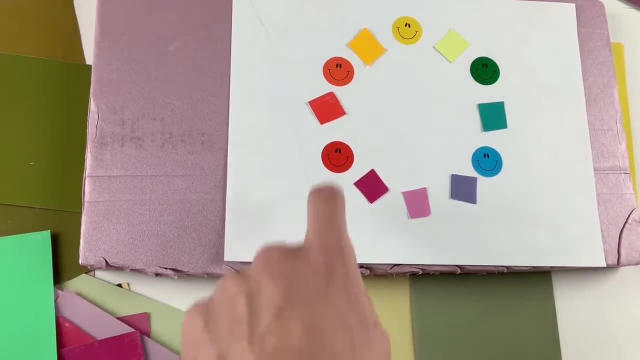 a red orange. I'm not sure if it's gonna be red, violet and I can experiment with those colors once I get there. so I'm gonna put my eyes on the red orange and put this one. I'm gonna use red or red, violet here: a red orange, red or red. 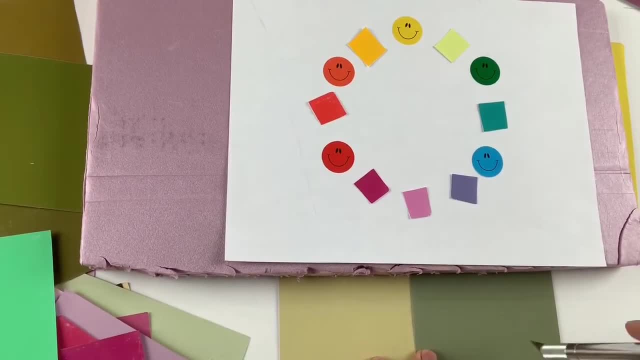 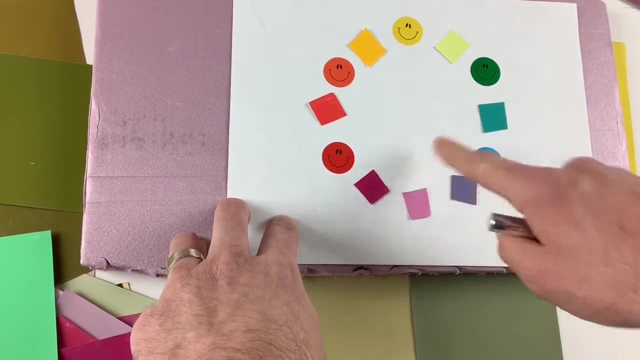 violet behind this guy, now this one, I'm trying to appear to make yellow, so I go up to yellow. what's the opposite of yellow violet? so now I know that this is the general direction where I want to work in. okay, so do I want to go to blue? 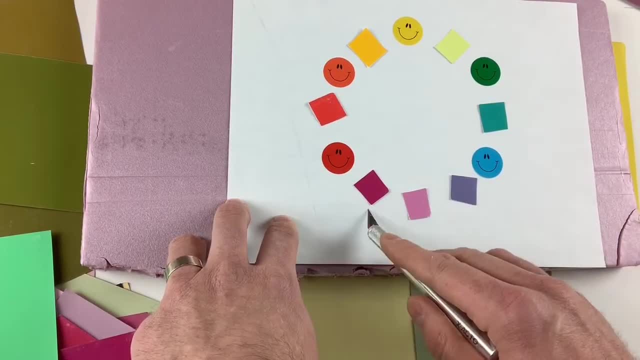 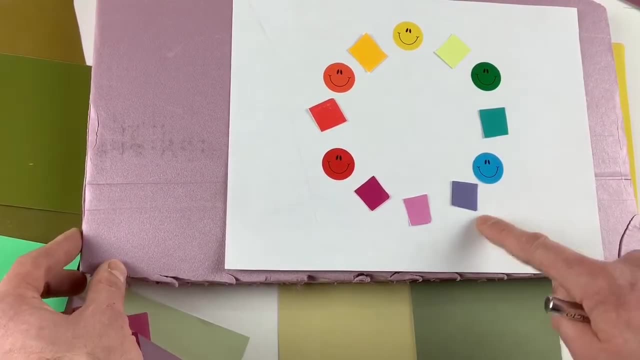 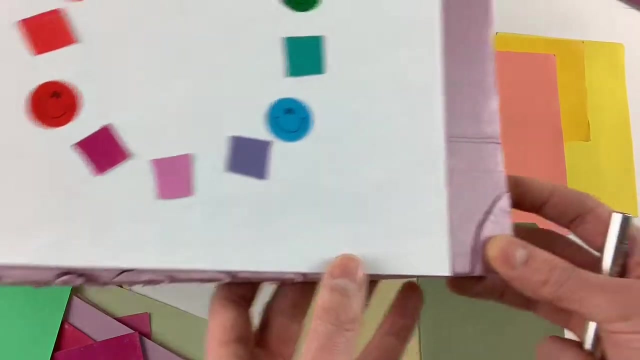 violet regular about, or red violet. I'm probably not going to go towards red violet if this guy is also red violet, because it would be doing the same thing. okay, I might end up over here, and I might end up over here in terms of the background colors that I'm going to select. okay, the other thing I need to 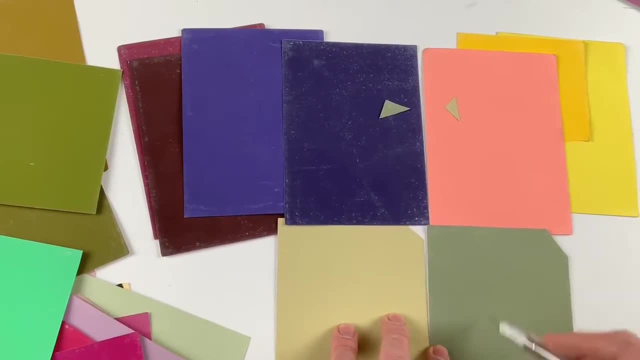 consider is: I need to make this lighter, I need to make this darker. so whatever I choose, if I'm making this lighter, then I'm going to choose a dark value. by making this dark, I'm going to choose a light value value. all right, so I'm. 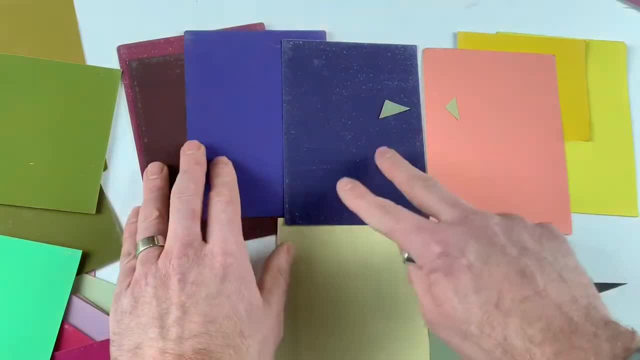 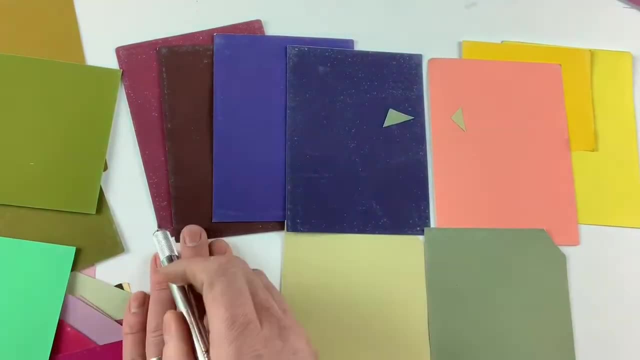 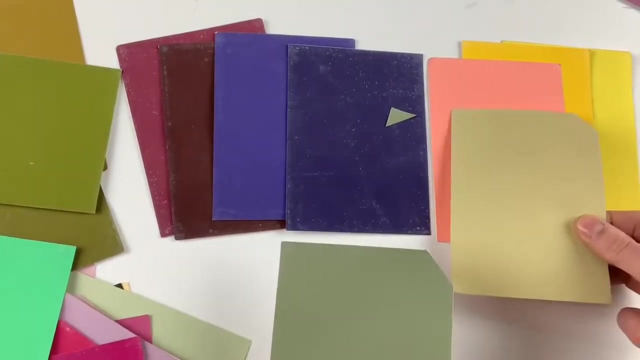 going to choose a dark value and what I have chosen here. if you can see, I experimented before I made the video and you can kind of see my trail of colors that I chose. I chose a red, violet. these are all dark values, for I go any further. 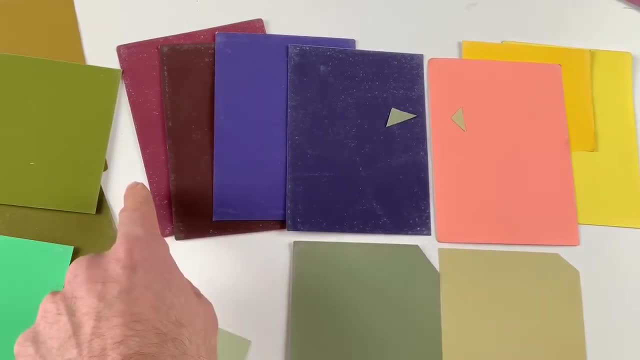 this is the same color and this is the same color. I'm just gonna flip these so it's not too confusing. these are blue violets or blue violet, dark blue violet, Red violet, red violet with more chrome. I tried all these and this one seemed to be the best candidate. 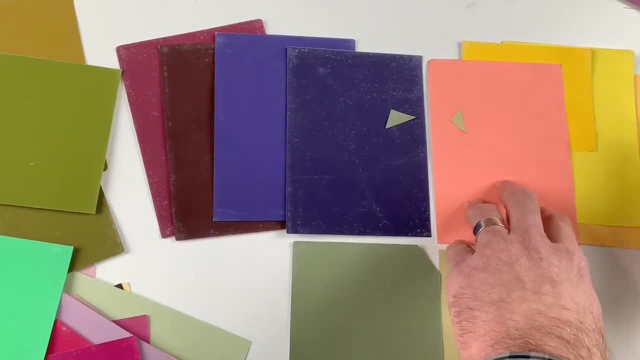 If you can kind of see my colors here, I tried a variety of colors. I tried this red-orange, very light in value. I tried just a pure yellow, Just out of curiosity to see what it did. I tried this other red-orange that had a little more yellow in it. 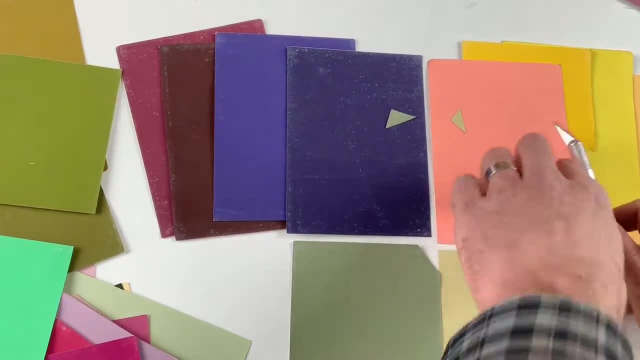 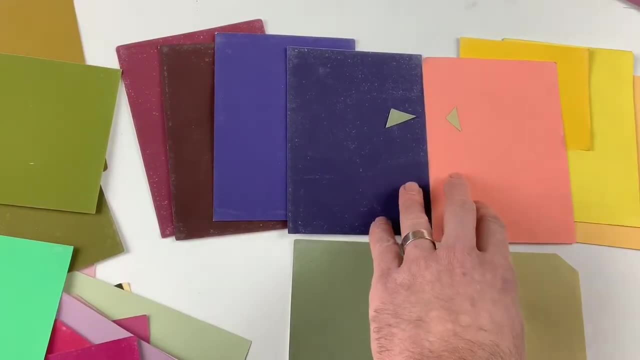 And then I tried this kind of peachy color, if you want to call it that, But it's basically a tinted red-orange, And this seemed to be the best candidate I could, maybe if I found something slightly lighter than this. 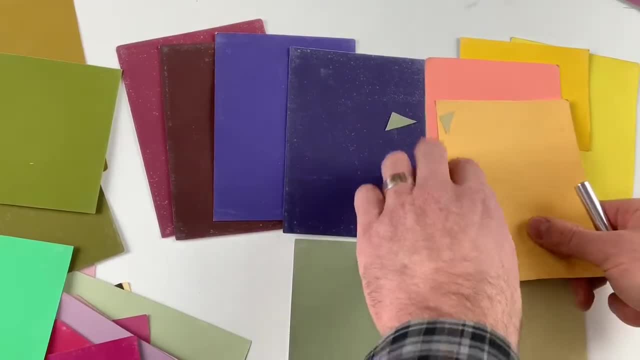 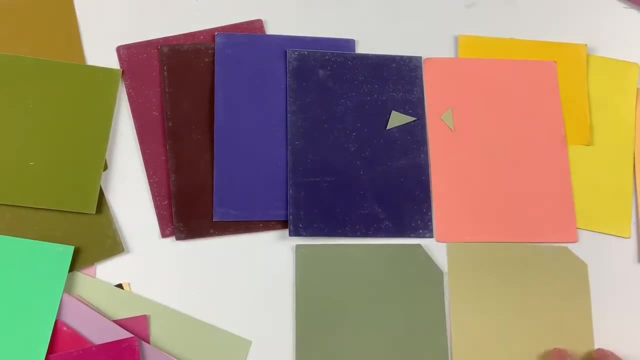 I could probably get that value a little bit more accurate, But once I put this behind, you can see where it becomes more gray. So I think the red is helpful to make it appear more green. Now I chose a lighter value, obviously because I need to make this appear darker. 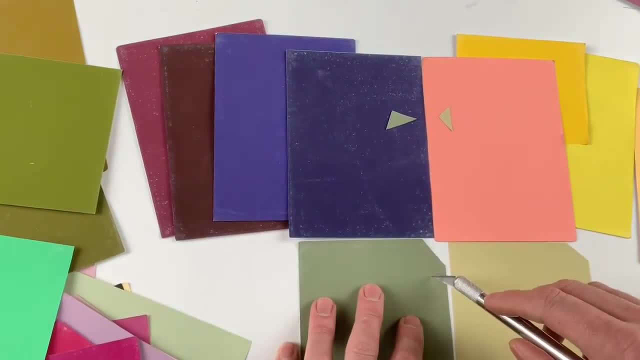 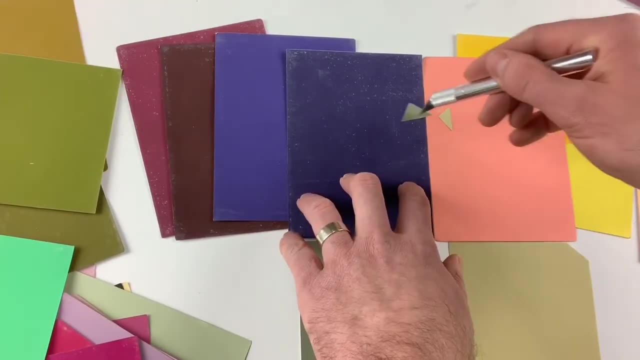 And I chose a darker value because I need to make this appear lighter. So this blue-green Made this work. Now I'm going to flip these guys and explain a little bit further. I put this same color on this side. I put this on this side. 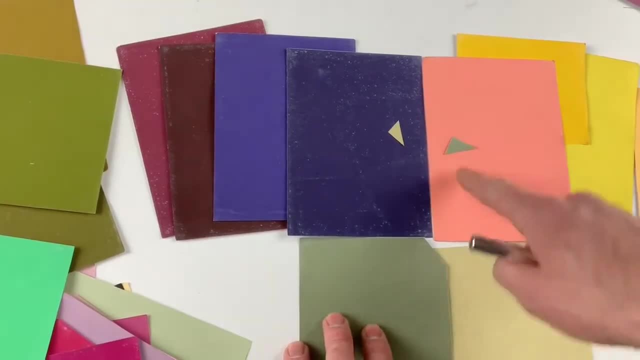 This color. I put on that side It actually, if you look at it compared to here, it looks more blue and it looks darker in value, Because the opposite of this is blue Color wheel, which is red-orange. The opposite of that is blue. 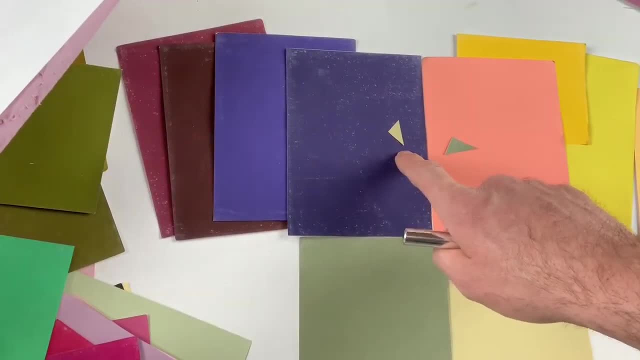 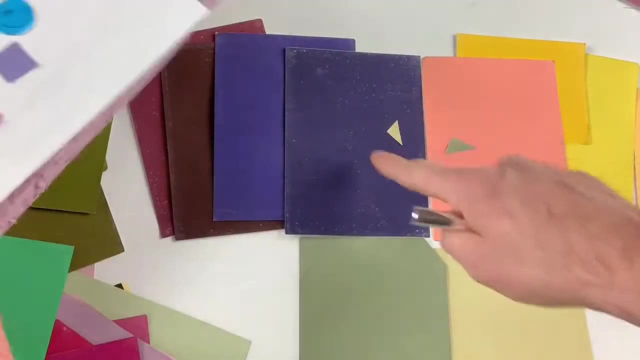 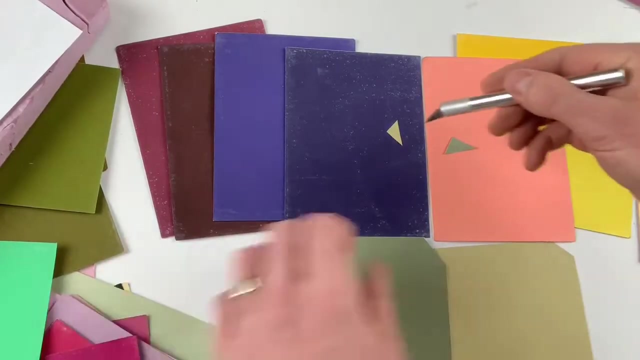 Right, This one appears more yellow. Why? Because there's a blue-violet underneath of it and yellow-orange is the opposite. So it just makes it's more yellow than orange. So it just makes this appear more yellow, But when I flip them back they almost appear to be the same. 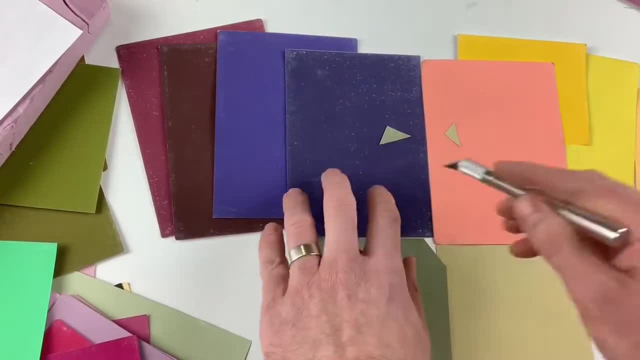 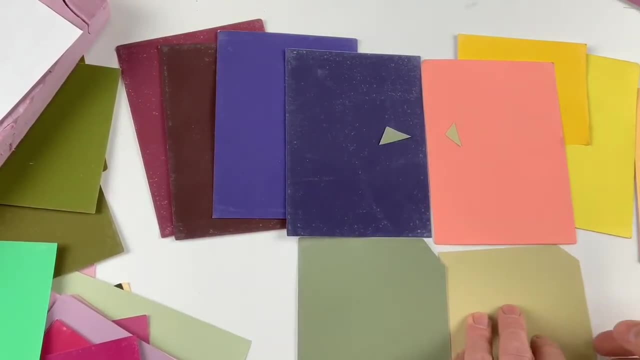 because the same concept is happening here. The opposite of this is yellow, So it makes this appear more yellow compared to what it is. The opposite of this is blue, And it makes this appear more blue, So it makes this appear more yellow compared to what it is here. 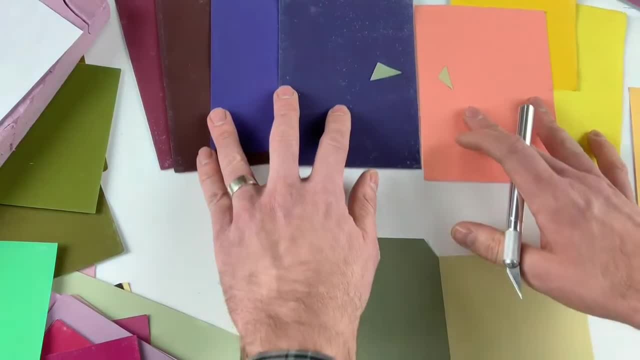 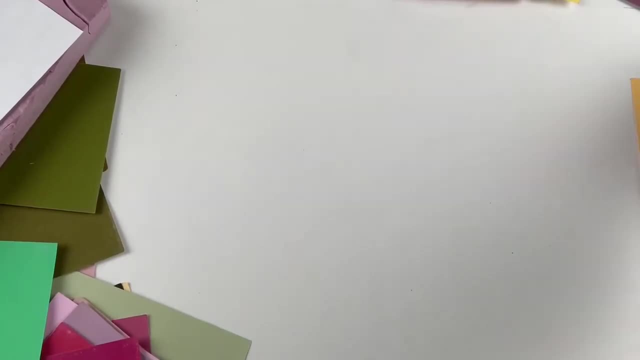 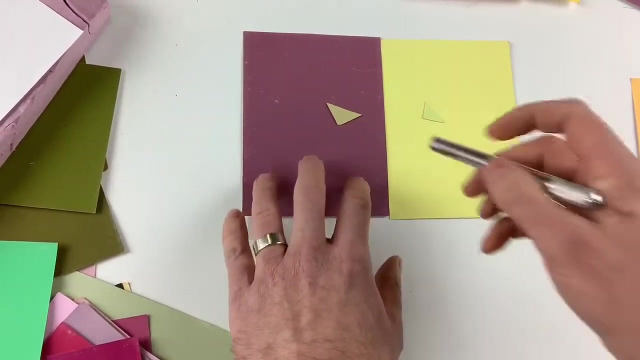 All right, I'm going to put this on the side. I'm going to explain one more example. It might be similar, I'm not sure yet, but there's a little bit of a. How does that look? Okay, So these two colors at first glance appear to be the same. 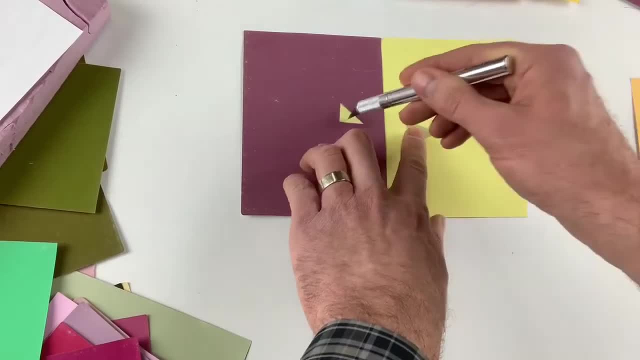 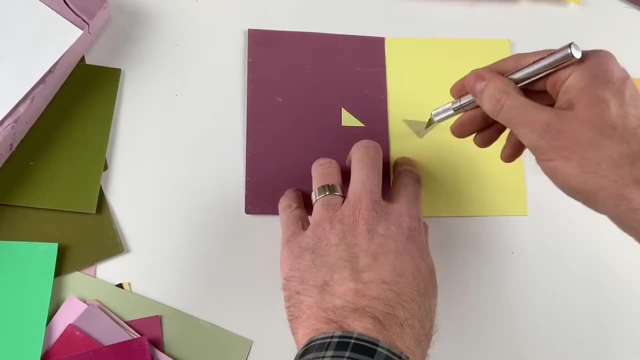 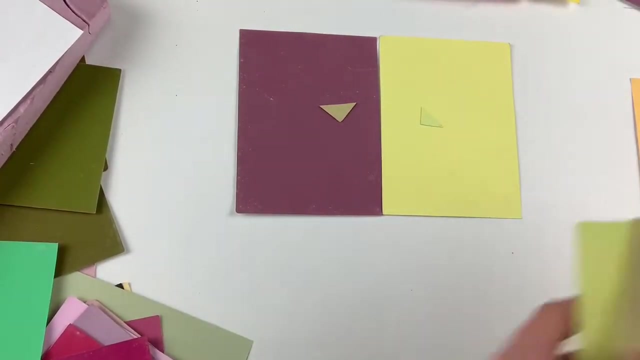 When I flip them, they're drastically different. Look how intense that color became. Now, I'm going to explain this in a second, but I have to show you the two original colors that I have. Okay, So here's the two colors that I'm trying to differentiate between. 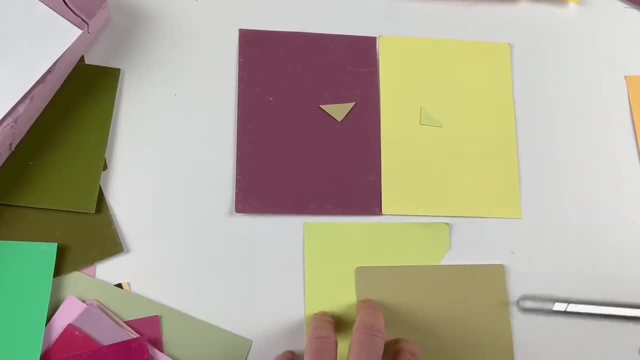 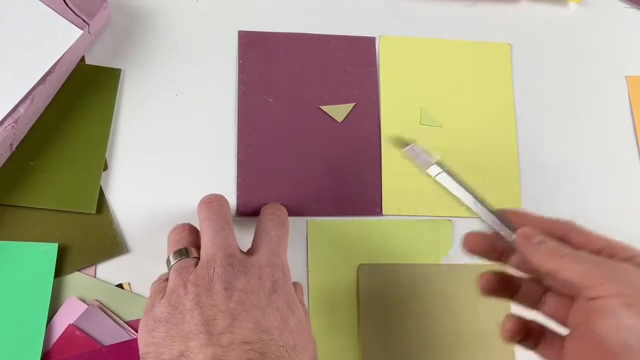 All right. So what's the difference between these In terms of hue, value and intensity? Right, So contrast of hue. Let's talk about value first. This is darker, This is lighter. That's pretty easy. That's why I chose a dark one. 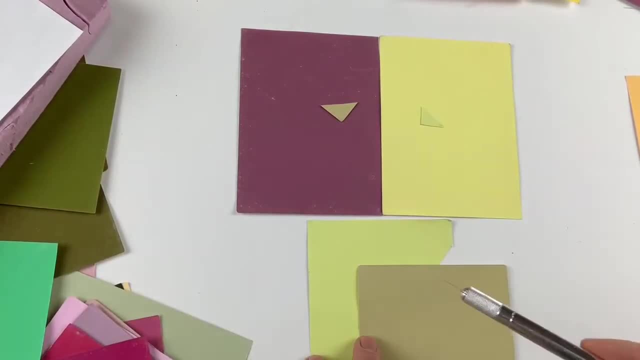 That's why I chose a light one, So I can make them appear to be the same. This one is much more grayed out than this one. This is very intense, And this is almost. It's not a pure gray, but it's grayed out. 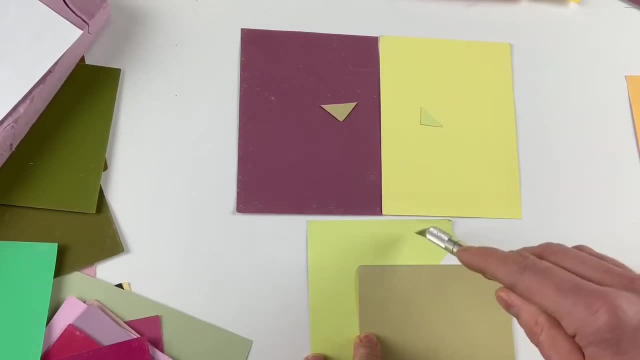 It's kind of like a middle to low intensity level. This is very intense, So there's a huge contrast there. So value and intensity In terms of hue this appears to have. This has green, yellow and green in it. This has. 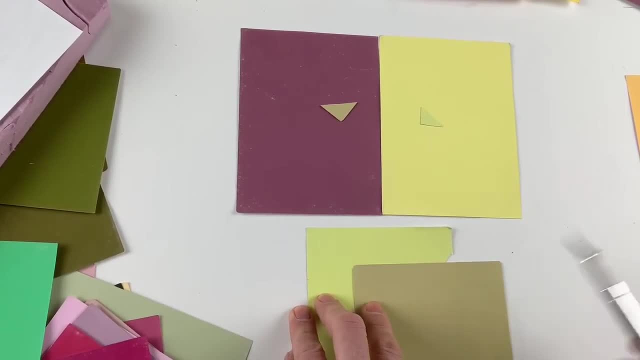 I feel it's more on the orange kind of. It has a little more orange in it. Okay, Now, before I even go there, I'm going to see if I can attack this without thinking about the hues yet. So I'm trying to make this color appear desaturated. 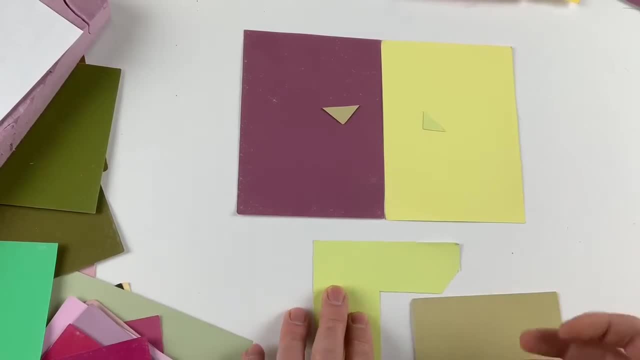 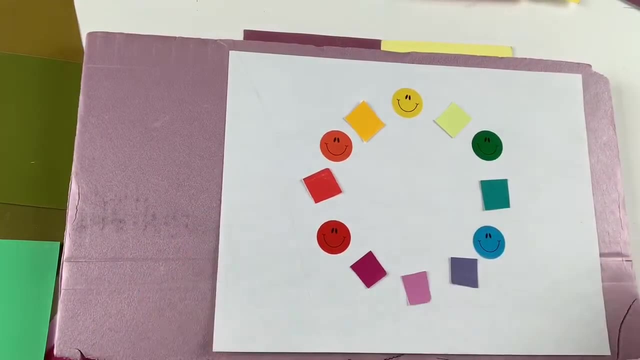 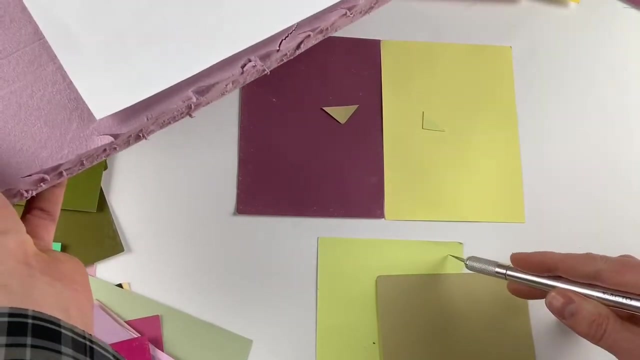 In order to make something appear desaturated, you have to put, You have to think of the hue or the color wheel here only because this is where it gets kind of tricky. So I'm trying to make this Again. I'm trying to make this color look desaturated. 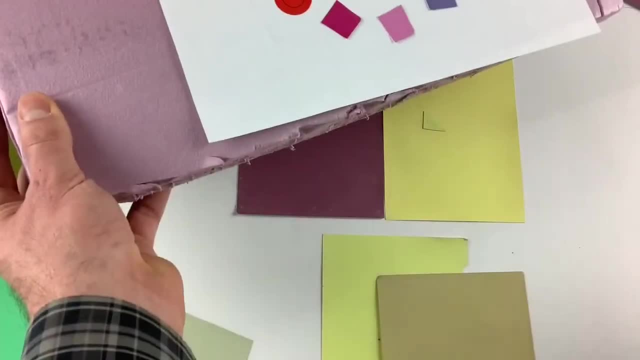 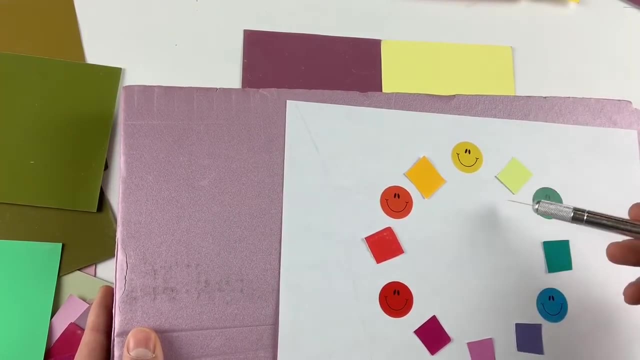 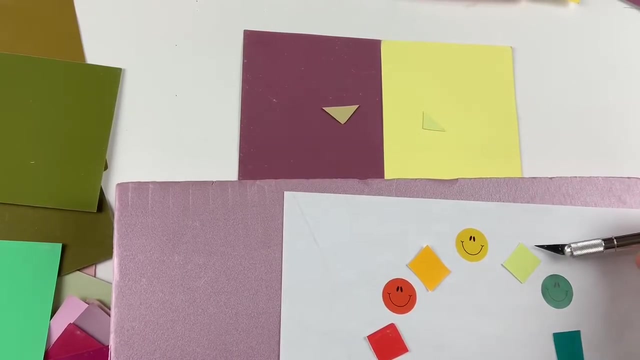 And this is a yellow-green right. It comes from this area here. I actually think that's what the color is. It's a yellow-green, And the opposite of yellow-green is red-violet. But when you put an intense version of itself, 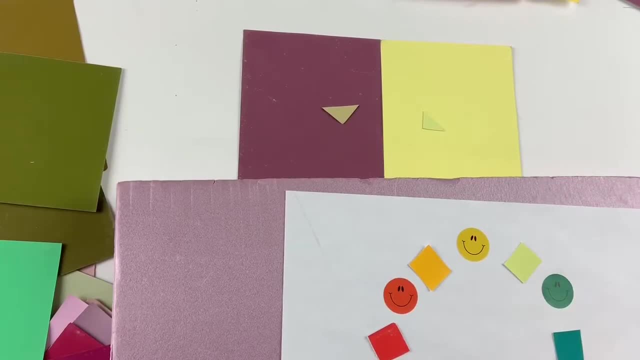 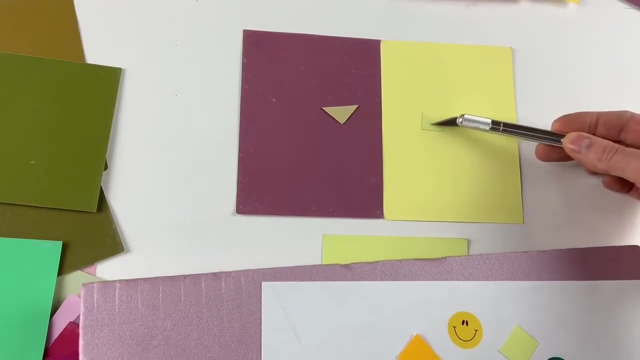 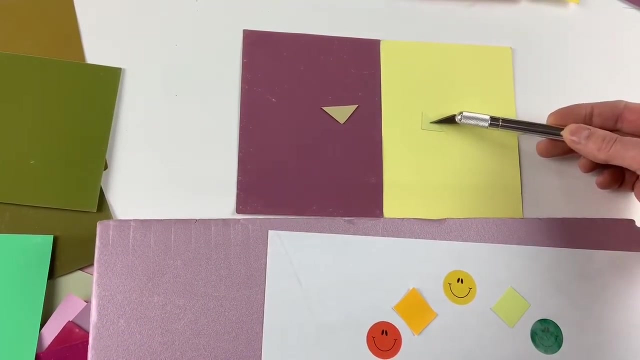 behind itself, it will create this cast. So, for example, I put this kind of intense yellow-green behind it and it made this appear grayed out only because the opposite color of yellow-green is violet. So violet is visually mixing with your eyes. on top of this, 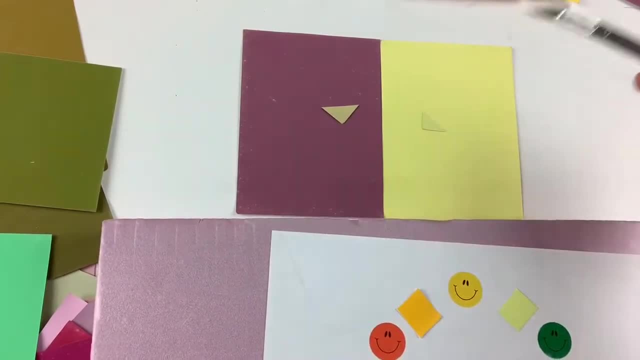 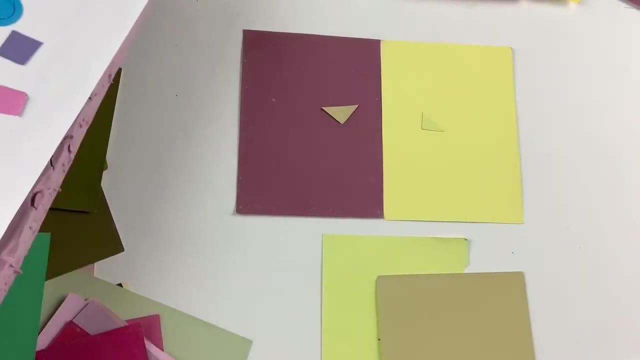 and it appears to gray this out just a hair, just slightly, just enough to maybe It can start to appear to look more like that guy on top of this background. Now I'm trying to make this one appear yellow and lighter in value.